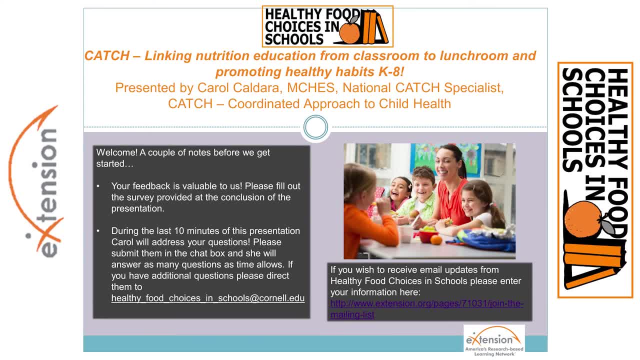 Good afternoon, everyone Welcome. Thank you for joining this webinar. It's presented by the Healthy Food Choices in Schools Community of Practice. Today we're pleased to welcome Carol Caldera, a nutrition specialist for the Coordinated Approach to Child Health Program, also called CATCH. Today she'll share with us how the evidence-based CATCH program uses a coordinated approach to nutrition, education and physical activity that creates and sustains a culture of school health. So thanks again for joining us. 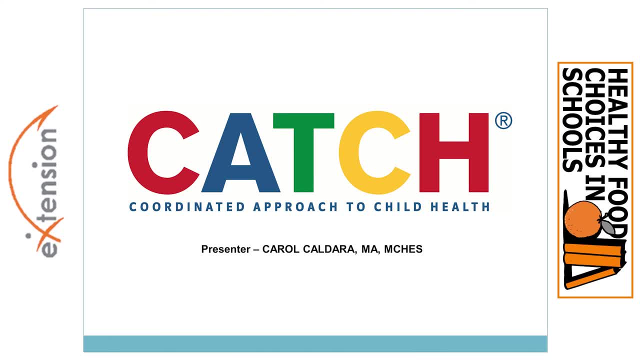 Here's Carol. Thank you, Katie, Thank you Extension Communities of Practice for hosting the webinar and thank you to Iowa State for providing technical assistance. CATCH is an evidence-based child health program that is targeting elementary school, middle school and also provides an after-school and a preschool program component. 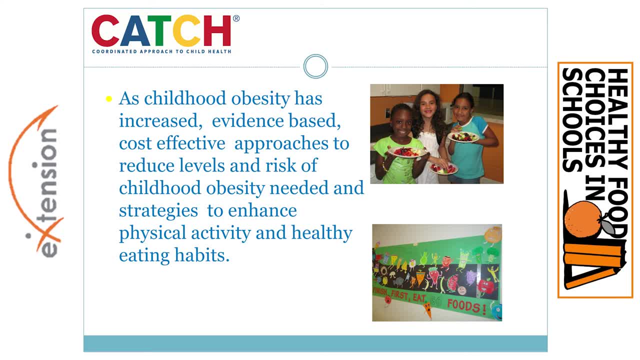 I would like to give you an overview of the program so you understand a bit of the history and how the program works. The program can now be applied to the work that you do and welcome everyone. Thank you for attending. As child obesity has increased, the percentage of overweight children in the United States has grown to a point where many really call it an epidemic. 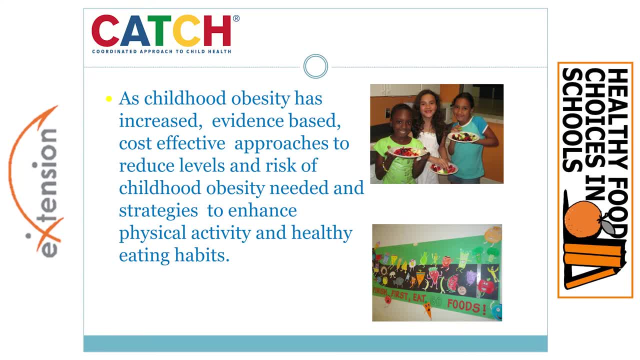 And overweight children, we know are at risk for health problems during youth and as adults. Overweight children and adolescents are more likely to have risk factors associated with cardiovascular disease, such as high blood pressure, high cholesterol and type 2 diabetes. 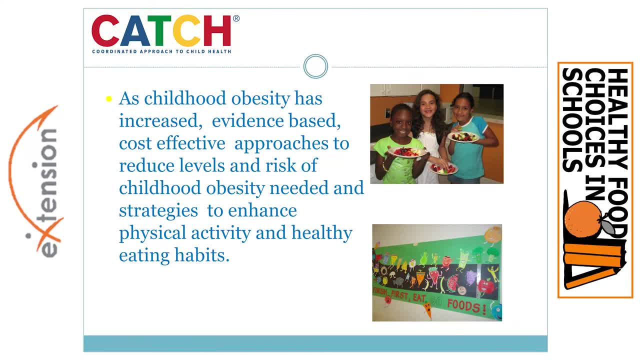 And overweight children and adolescents. And overweight children and adolescents are also more likely to be obese as adults, with studies showing approximately 80% of the children who were overweight at age 10 to 15 will be obese adults when they reach 25.. 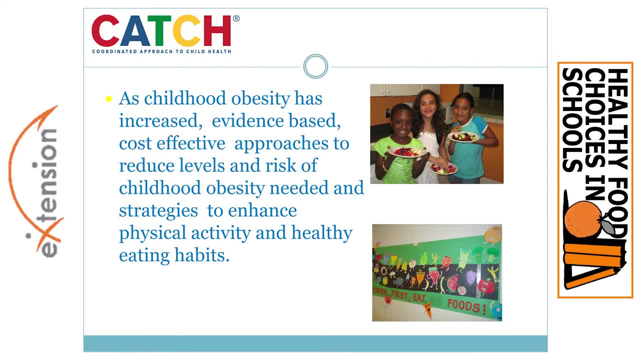 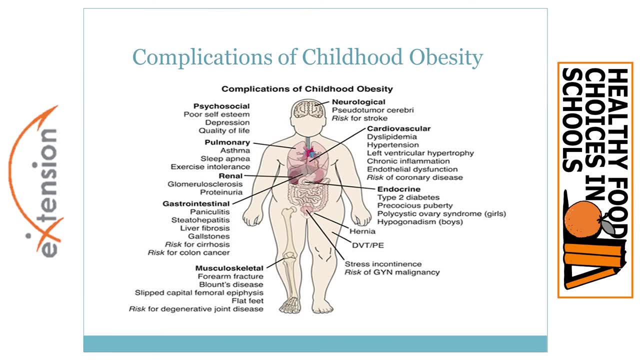 Evidence-based approaches are really crucial, and prevention of child obesity is crucial and is an upstream approach. Here we have some of the complications of child obesity and there are many, Many detrimental consequences can occur. Type 2 diabetes is commonly referred to. 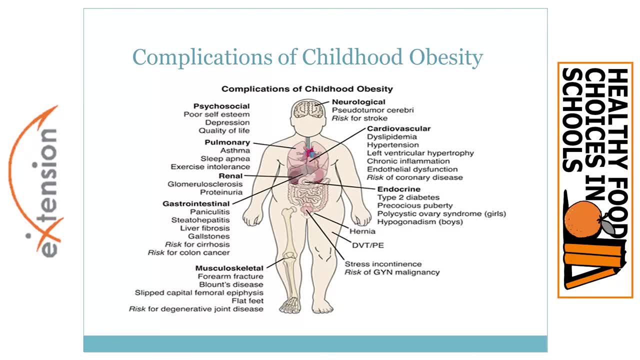 As adult onset is happening with much more frequency in young children. as obesity rates soar, there is a correlation. Other negative physical and psychological impacts and risk factors can increase with child obesity and is very costly to the health and the future of our nation and to the health of our population. 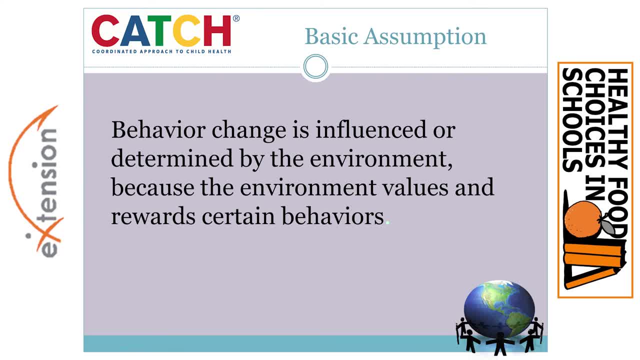 So we begin with a basic assumption: Behavior changes influence or determine by the environment, because the environment values and rewards. If a child is Sod-free or obese, there is a correlation to age, age become key. So what we can do to help us understand the impact and damage behavior can be. 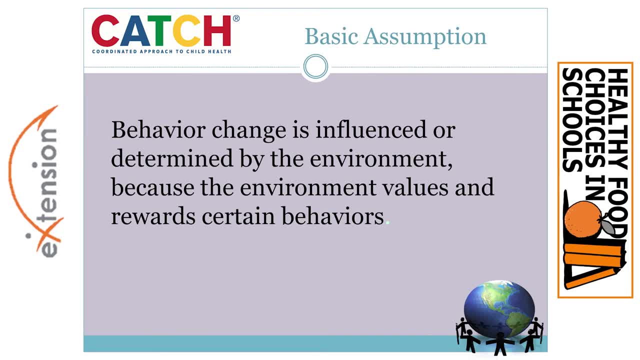 How can we improve behavior? Do you think that we should change behaviors towards certain behaviors? Would you agree? Stated another way, in today's society we act possibly a little different than we did 20,, 30, or 100 years ago, because our society is different and changes. It changes slowly, with cultural norms and expectations that influence behavior and things like values, role model, information, studies, the media and expectations are some of the factors that slowly impact and change behavior. So we begin with a basic assumption: Behavior changes influence or determine by the environment. 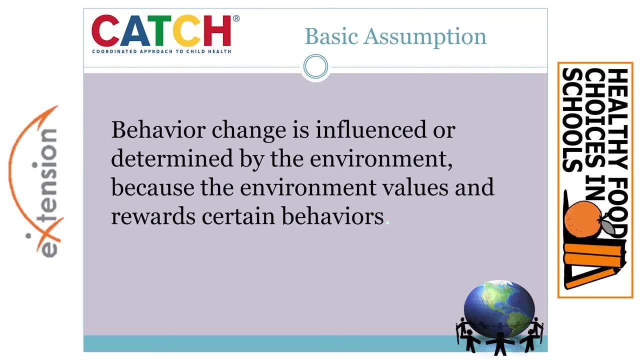 So we begin with a basic assumption: Behavior changes, influence or determine by the environment. Things like consumer behavior can cause a growing risk of diabetes, And things like values, role models, information, studies, the media and expectations are some of the factors that slowly impact and change behavior. 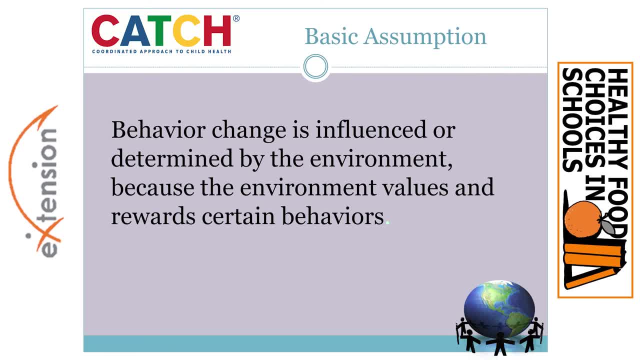 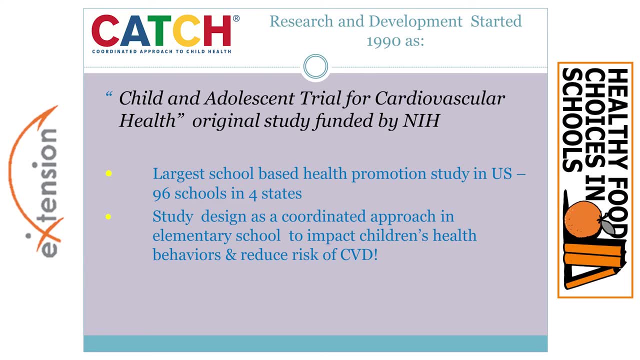 So it's very important to value health in our society. CATCH was the largest school-based health promotion study that was ever done in the US. It was funded by the National Institute of Health and four US universities collaborated. The impetus to begin CATCH was to reduce risk of cardiovascular disease and CATCH succeeded in producing lasting changes in dietary habits. self-reported physical activity behaviors. 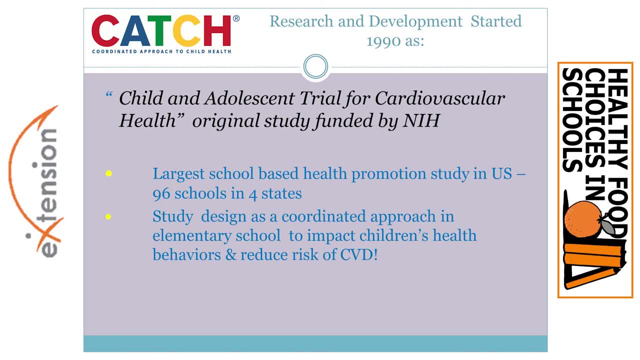 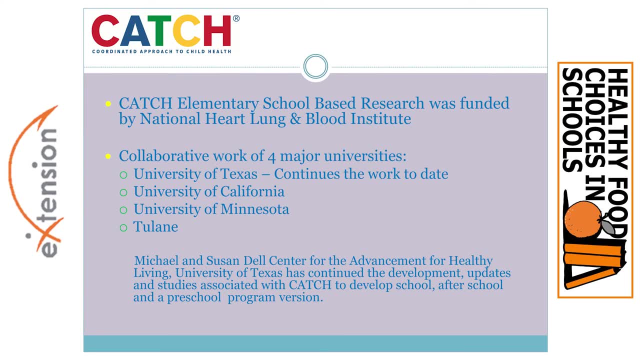 and students who participated in CATCH also consumed less fat and participated in more physical activity outside of school. Here you see the universities that collaborated- University of Texas, California, Minnesota and Tulane- in the original CATCH trial that lasted several years. 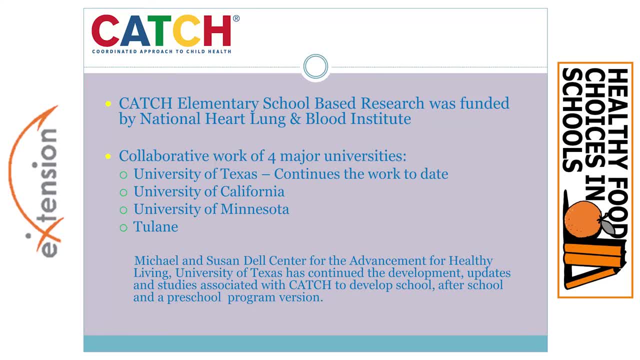 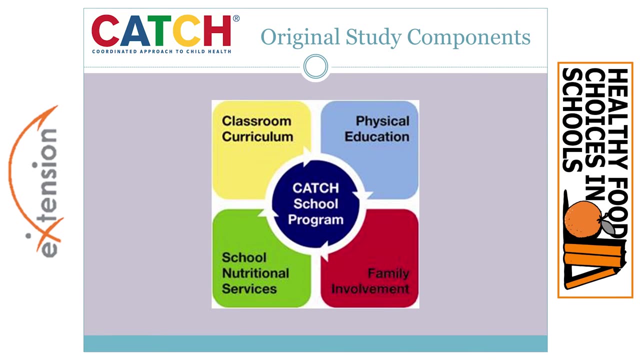 And ongoing. the University of Texas and the Michael and Susan Dell Center Advancement for Healthy Living has continued CATCH development and research going on now about 25 years, and they've had many positive outcomes. The original CATCH components, and still included in the current program for schools, include a PE program that's very moderate to vigorous. 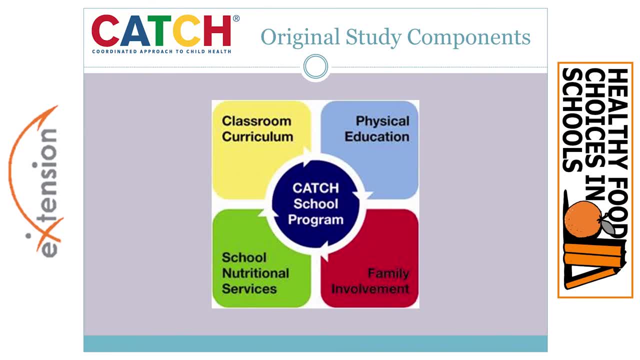 and Eat Smart component, which is actually the school nutrition. The new CATCH program includes a health and wellness service guide and includes cafeteria and the directors and staff. The family is involved and in classroom curriculum with nutrition and health. So there's multiple components and we now also have included new CATCH coordination guides that help to improve the school health environment. 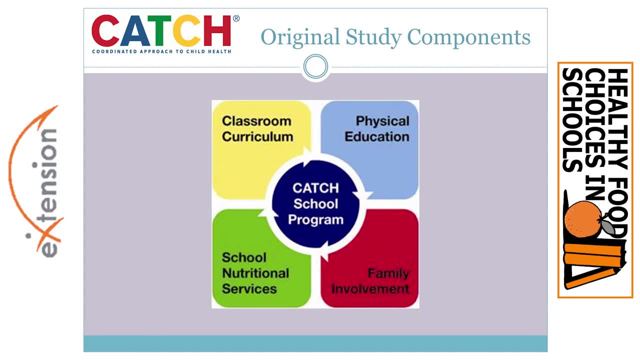 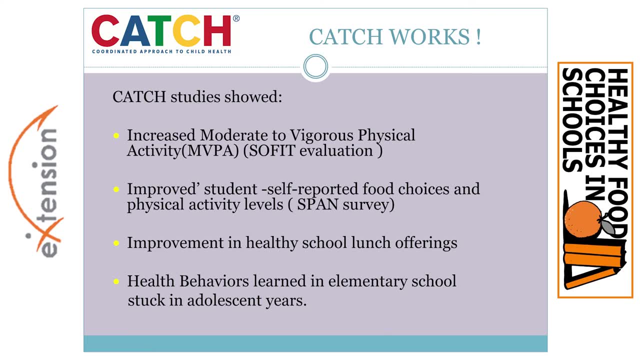 and they include elementary and middle school coordination guides for campus-wide healthy messaging. So the original CATCH trial, which happened in the 90s- we were able to reduce fat in the school. We were able to reduce fat in the school And guidelines for nutrition we know have changed. 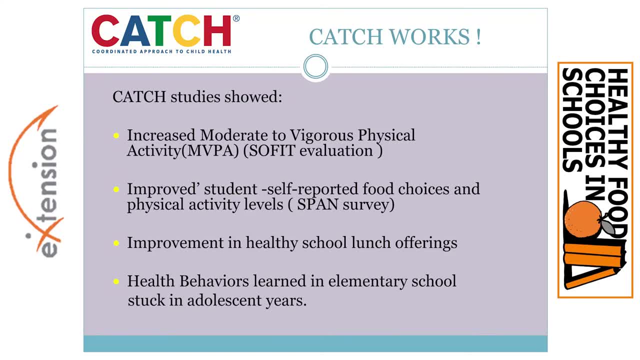 So as that has changed, curriculum and guidelines in the CATCH nutrition curriculum have changed. with the updated nutrition guidelines We were able to increase activity in PE classes and also children themselves reported to us they were eating and being more physically active at home or out of school. 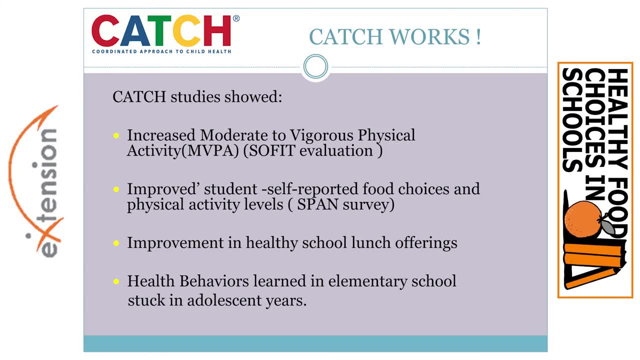 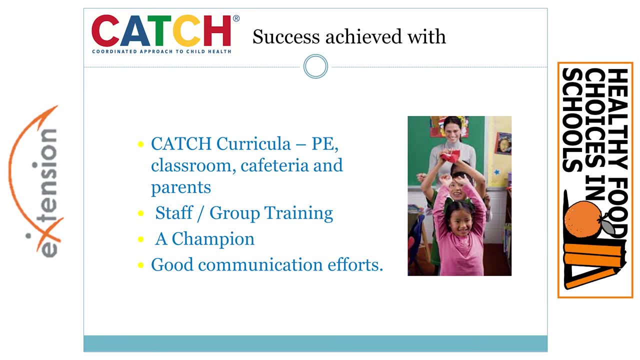 A neat thing about this is also that these behaviors were maintained even after the study was over and students were able to eat, and they were able to eat, So that's a good thing. went on to middle school. That was a follow-up study done to see if it stuck, which it did. 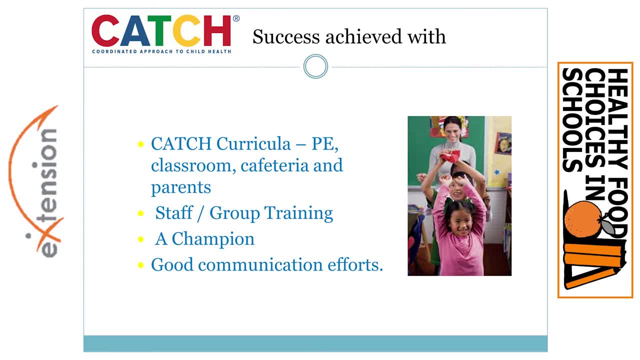 Planning for successful catch program implementations require a few things. It requires a catch team of several people and a catch champ to really take the lead. Knowing your target audience is important. Who are you working with And recruiting personnel and sites to implement the program is important to set your budget and plan to order catch curriculum needed equipment. 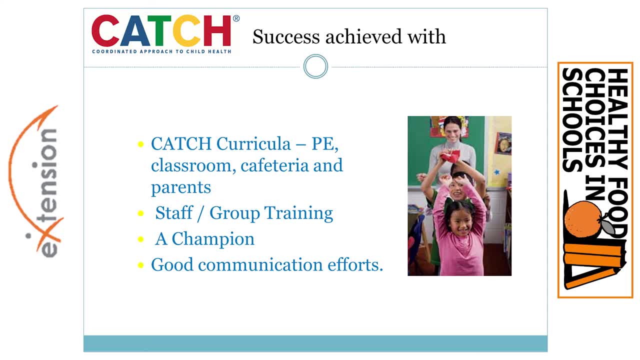 And training is very crucial. We now have several types of training, which I will go into a bit in detail, And it's important to gather some data. We have evaluation tools and components that can be utilized, that were utilized in the original studies, that can also be utilized in your. 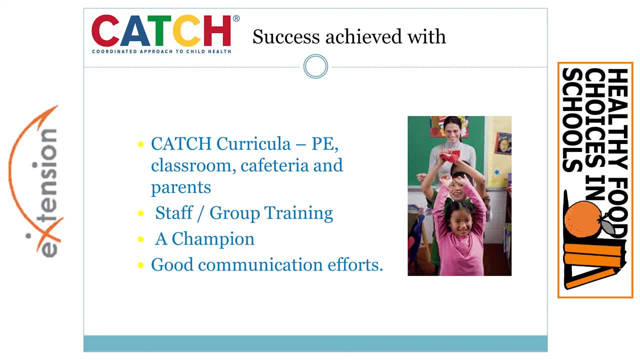 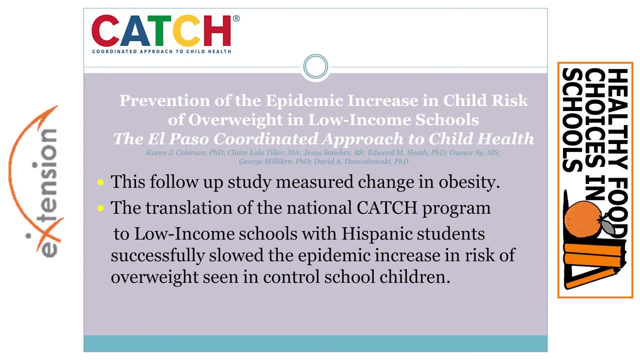 programs as a guide or verbatim, And good communication is important to now establish catch program in your area. Another study, a follow-up using catch, was a study that called the Prevention of the Epidemic: Increase in Child Risk in Overweight in Low-Income Schools. 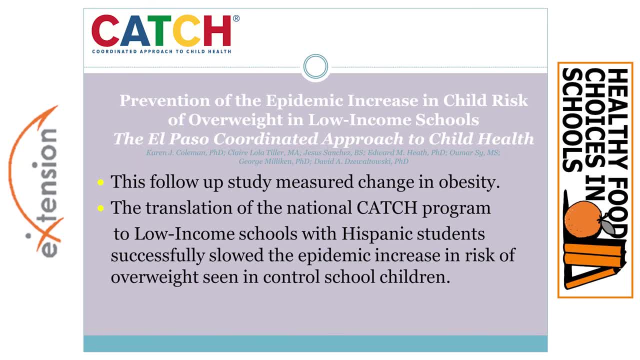 It was called the El Paso Coordinated Approach to Child Health And this particular study was a follow-up that actually measured obesity level change. So we know that in this particular study, which was quite a long term of the use of catch, it actually brought down obesity rates, while in 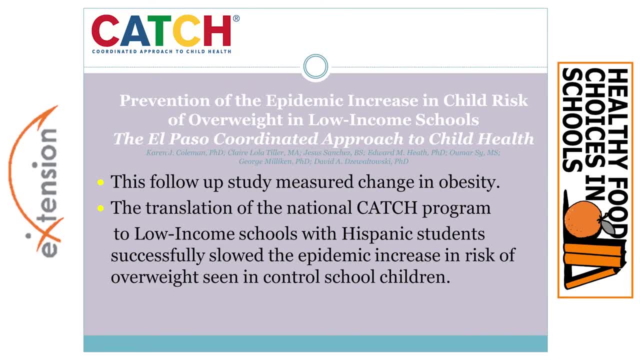 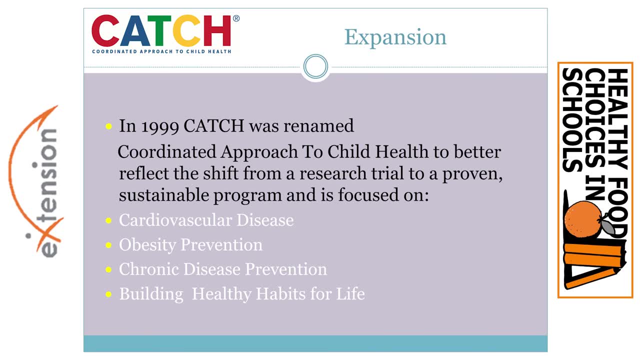 other counties other than El Paso, the rates continued to increase. So after the first initial assessment, and all in 1999, catch was renamed the Coordinated Approach to Child Health to better reflect the shift from a research trial to a proven, sustainable program And the 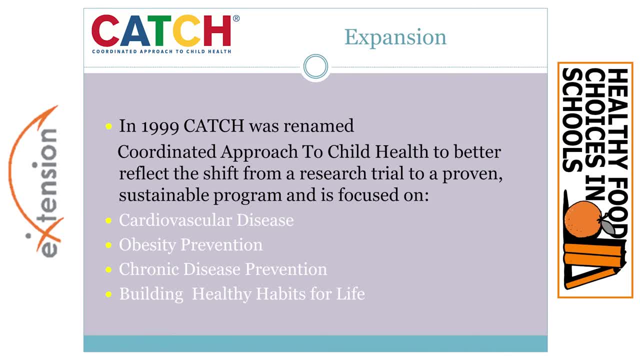 Coordinated Approach to Child Health also mirrored the CDC model that came out for coordinated school health with multiple factors to be included in a school. So catch now is focused on obesity prevention and cardiovascular reduction, chronic disease prevention and building health habits for life. If we can build healthy habits for life, we reduce chronic disease. The program 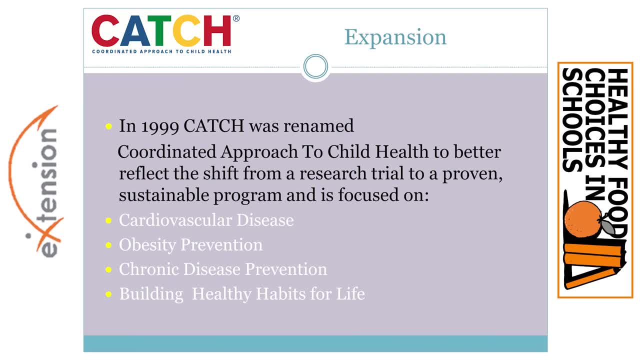 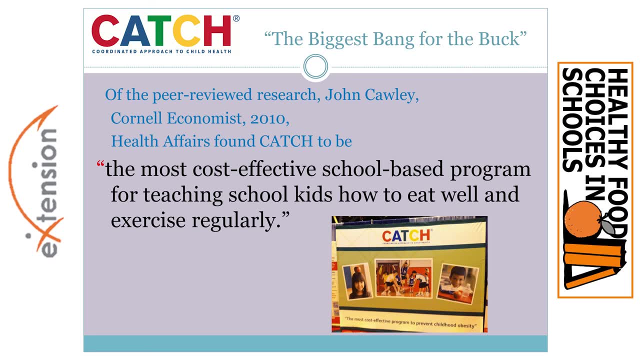 has now been implemented successfully in thousands of schools, both nationwide and also in several other countries. There is an economist named John Qualley and he's a Cornell economist and he did a review of programs impacting obesity that were utilized in schools And he found 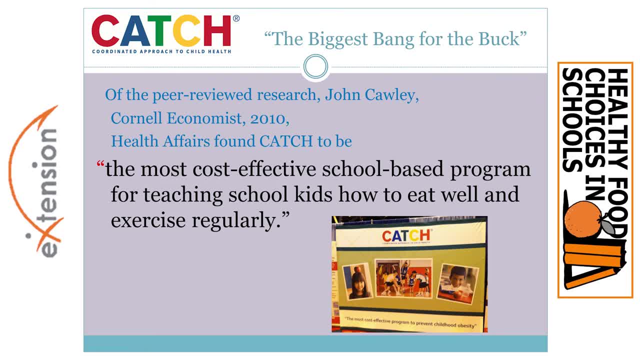 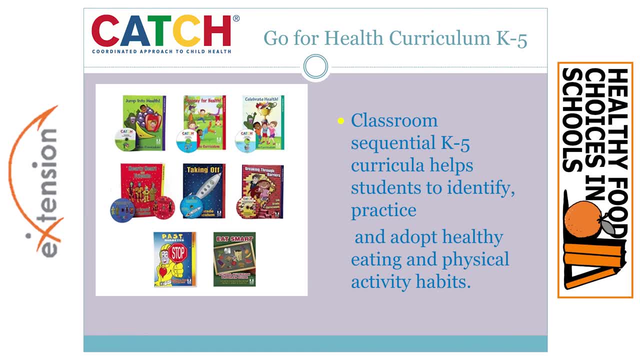 program for teachers And he found actually that the catch program was the most cost-effective school-based program for some nutrition concept with physical activity, some nutrition concept with physical activity. Here you have a slide of the Go4Health curriculum, which is the K-5 sequential grade. 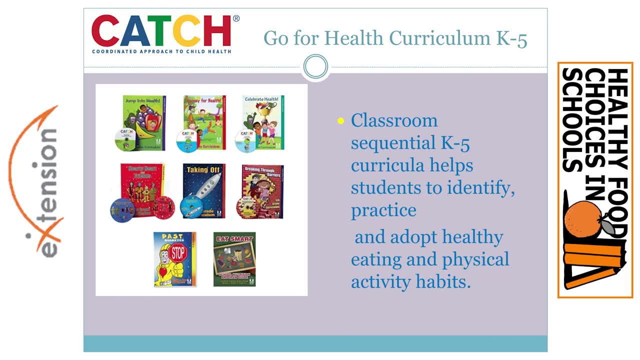 by grade curriculum. You can utilize this whole K-5, or you can actually zero in and choose one of the curriculum if you're working with a particular age or class or group. It includes a variety of learning methods, such as cooperative learning, discussion groups, individual. 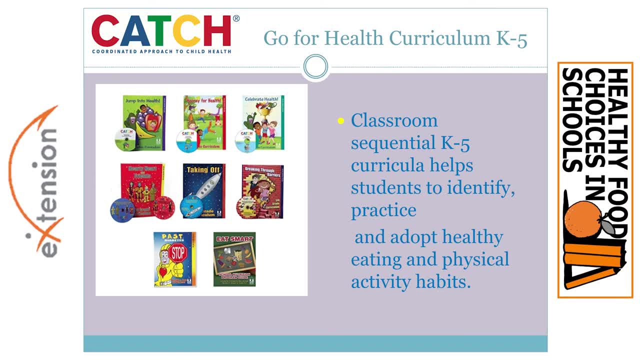 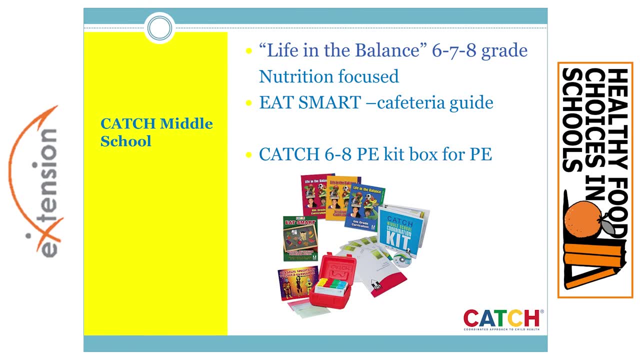 goal setting, reinforcement, skill building, a layout of games and adjustment, in addition to a variety of support from the Italian organization for guidance and development. addendums to do outside or extra. The middle school classroom curriculum is called Life in the Balance: 6th, 7th and 8th. These consist of classroom lessons of about 20-minute parts. 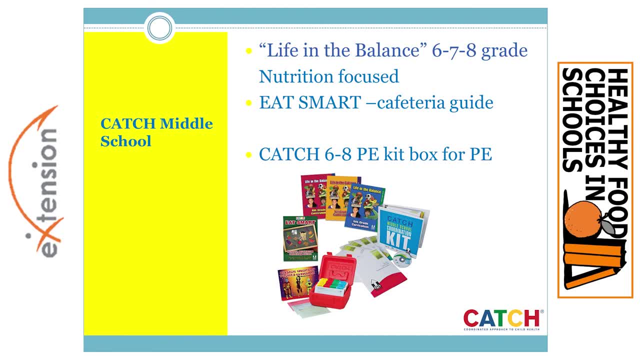 They can be taught. There's actually. one full lesson is about 40 minutes. They can be taught as two 20-minute parts or a full 40 minutes. The curriculum is designed to serve as a resource to supplement or replace components specific to nutrition and physical activity Curriculum. 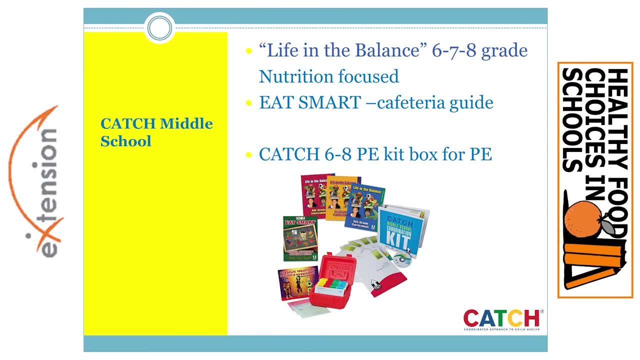 does not include specific tests or grading, It is recommended to evaluate on participation, skill building and some behavioral outcomes In the 6th to 8th. there's also a PE curriculum kit box And, as I mentioned, the school nutrition service, or cafeteria, is an integral part of CATCH. 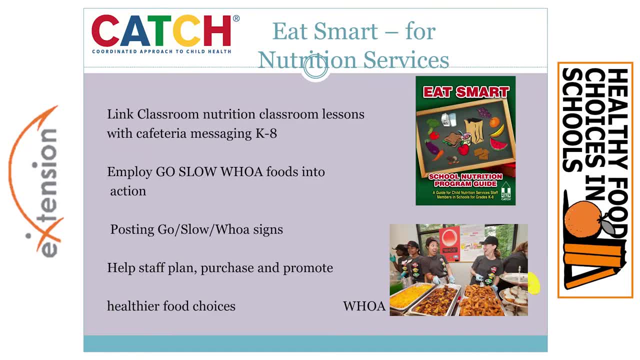 So the Eat Smart Guide that you see pictured links classroom nutrition back into cafeteria. It has cafeteria messaging all the way from K through 8. It employs go slow woe food messaging into action And I will tell you more. Go slow, woe is a message and a help to children on how to differentiate. 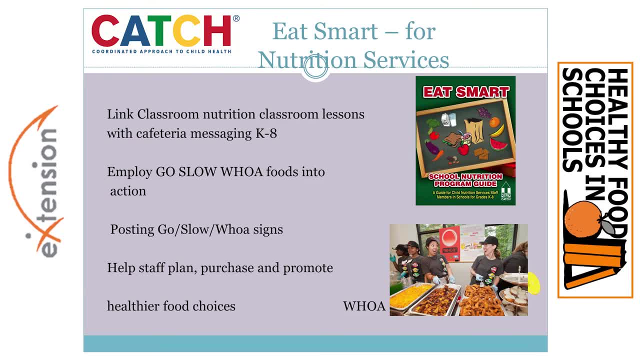 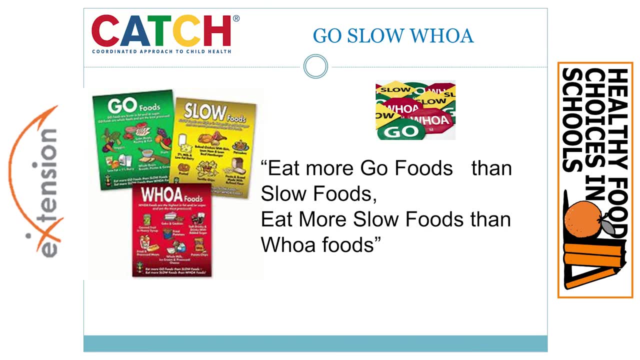 which foods are healthier than the next. The cafeteria can post go slow woe signs. Eat Smart Guide helps staff plan purchase and promote healthier food choices. The go slow woe concept takes all the foods and divides them into categories and go. 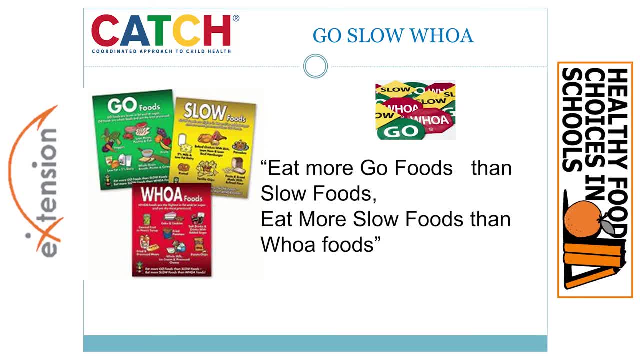 slow and woe Go foods are actually whole, untouched, unprocessed. The goal is to eat more go foods than slow foods. Slow foods are slightly more processed or added salt and sugar or fat, And woe foods are the highest in fat, salt, sugars and processing. There's 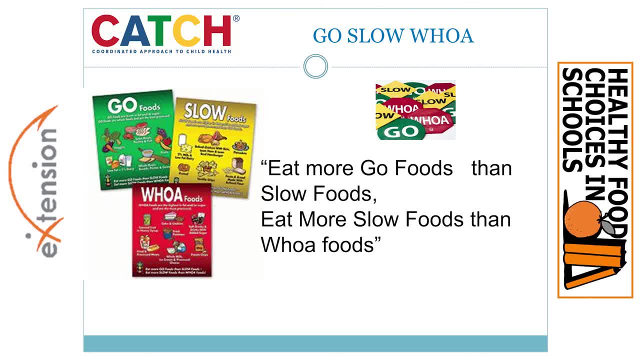 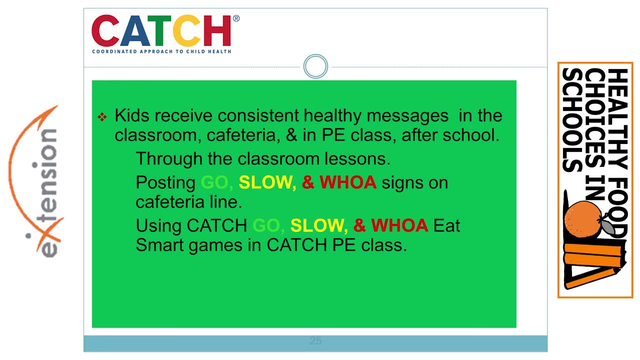 many tools to reinforce the message available, both in the nutrition lesson curricula as well as in the school cafeteria, as well as even sending those messages home. A CATCH goal is to promote the language and continuously remind children of the go slow, woe message. 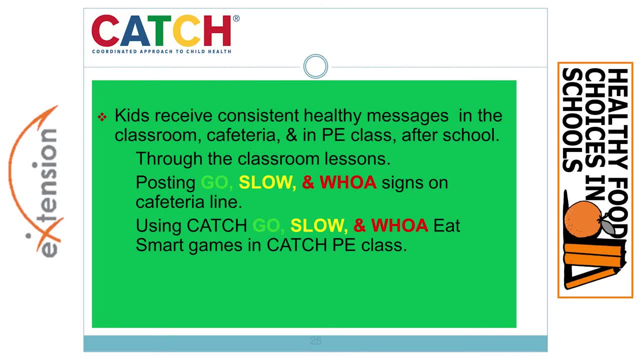 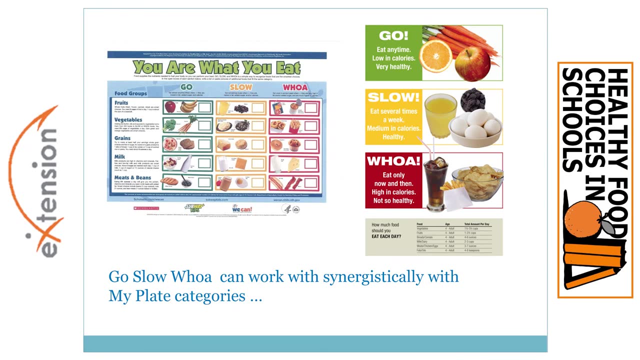 So there are many also, as I mentioned, integrating nutrition concepts into physical activity, And there's even some go slow woe physical activity games Connecting the cafeteria to other areas of the school, such as just outside the gym where you could hang various messages. 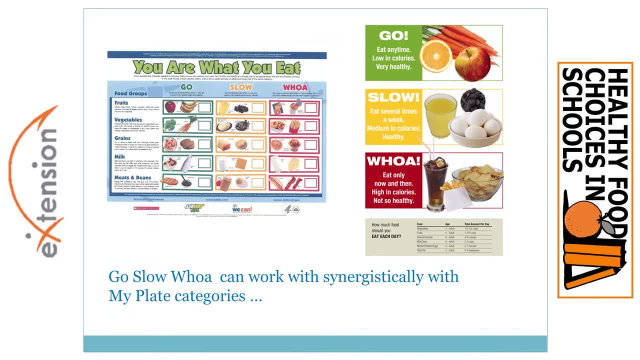 on healthy food choices. You can have poster contests and really, you know, help children understand We never say never, Don't ever. you know like no, don't ever eat a particular food. What we're trying to do in CATCH is to differentiate. 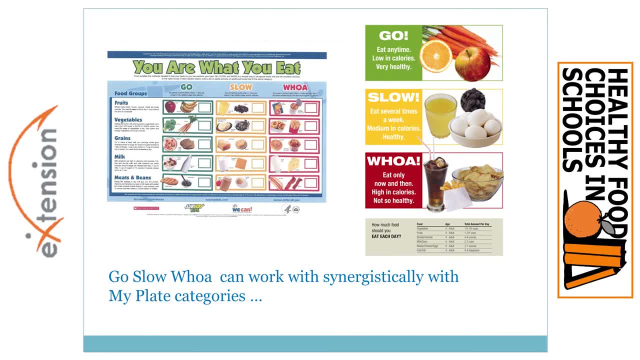 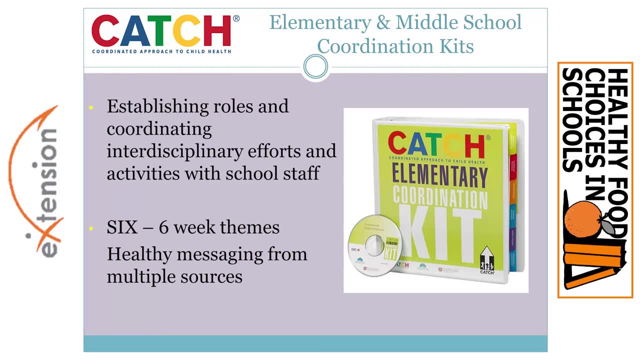 and help children know which food might be healthier than the next and working toward go. Another part of CATCH are the elementary and middle school coordination kits. These were developed later when, several years ago, federally, wellness policy became mandated And the CATCH developers and researchers realized that there 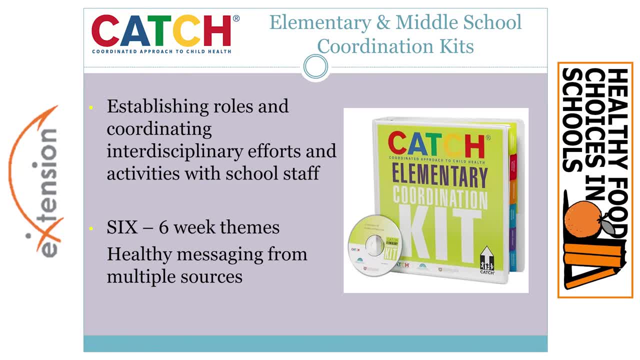 was a piece missing That was needed to help an entire campus, provide healthy messaging, establish roles and coordinate interdisciplinary efforts with their school staff. So there's an elementary coordination kit and there is a middle school coordination kit. They provide six six-week themes. So 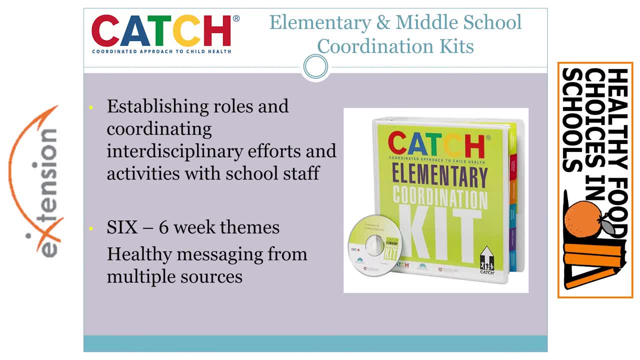 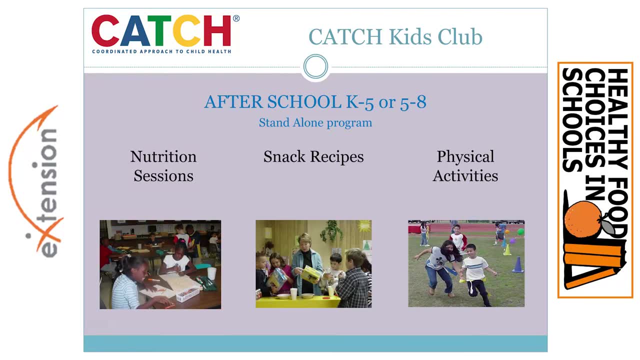 you can work through a theme and each department has their little piece to do. So that I just completed was more of the overview of the school-based portion of CATCH. The CATCH Kids Club is the after-school component, which consists of a nutrition section, a snack. 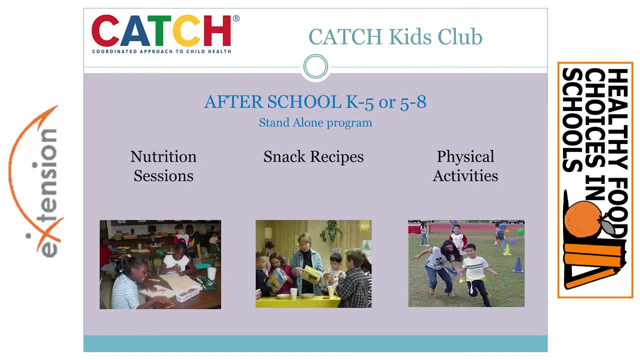 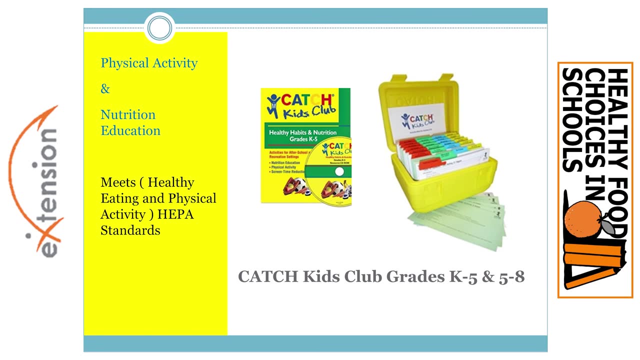 making and physical activity portion. You can use this as a standalone after-school component and it also has a K-5 or a 5-8 grade curriculum portion, And here you see the nutrition catalog or curriculum. And here you see the activity box that contains the physical activity. 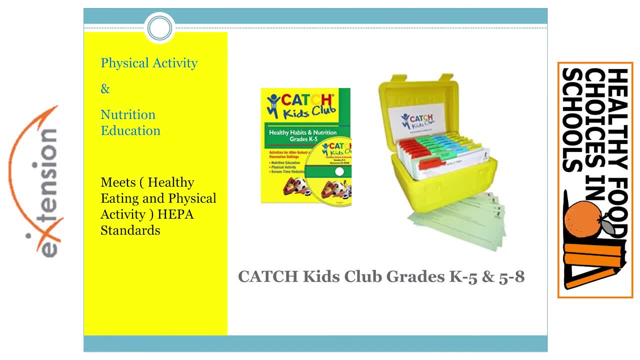 cards. CATCH Kids Club. we call that for the after-school. Now, some of the activities that we do include the physical activity cards. Some of the activities that the team did include the physical activity cards. And, as for the four-hundred, helping 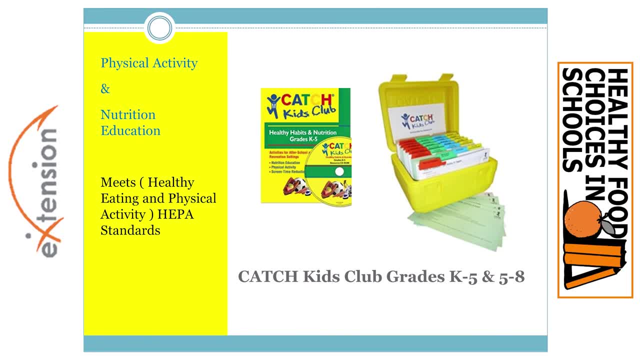 kids. you can really picture how they went through the круг, the single days And when there's a friend or a nossas and some of the other members who help them with this, and then you try somebody else's technique, then you try their technique and consider 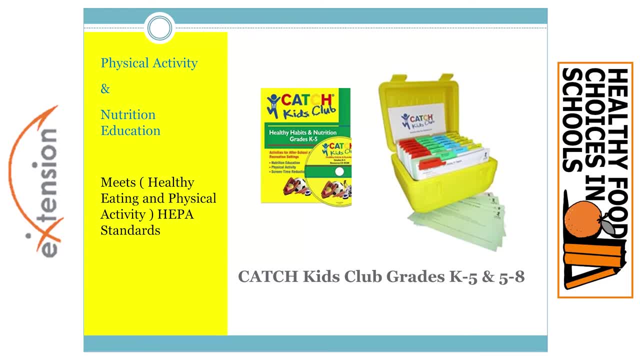 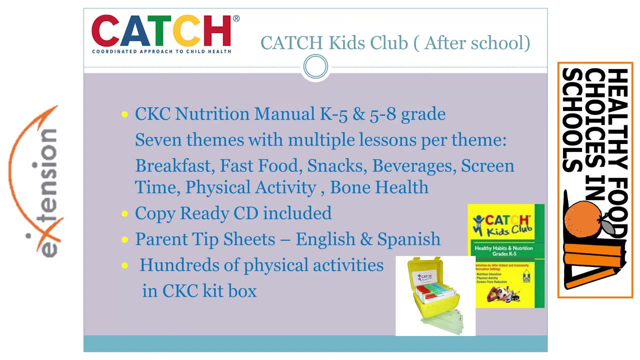 how they're doing. Then again, kids wouldn't. I think the bestREAM team would have to go PERS BIGONG to collaborate with certain universities and Resort andtó with individuals who want to get some experience conducting the physical activity. Definitely. 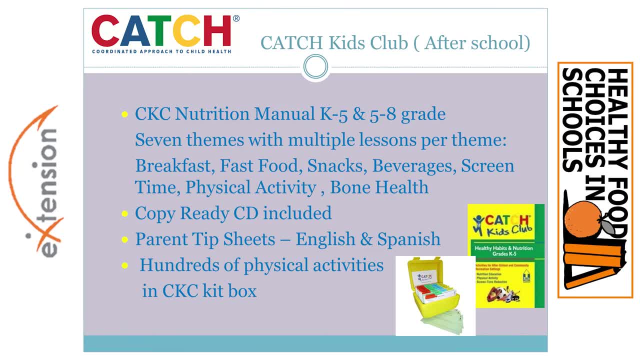 Thank you, guys for taking time out of your time. Thank you, Thank you, Thanks for winning, Thank you. It was found easy to use and a format that both children and staff enjoy. There's a snack-making portion after each group of lessons. 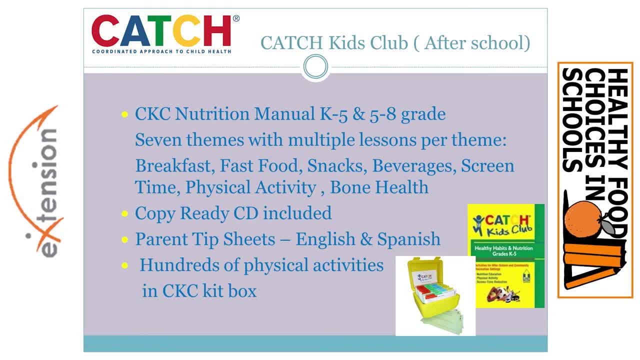 There are seven themes with multiple lessons per theme, and some of them, as you can see, cover breakfast, fast food, snack-making beverages, screen time, And there's also parent tip sheets and there's a nice copy-ready CD included in the booklet. 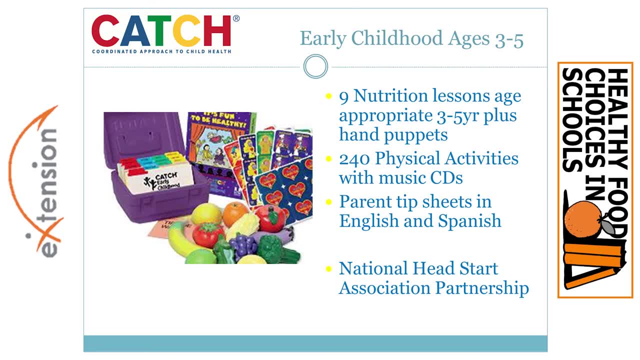 There is an early childhood section of Catch. I just want to make sure you are aware of that In the purple kit box contains 200 age-appropriate physical activities and the It's Fun to Be Healthy manual comes with nutrition and food garden lessons and it was approved by National Head Start. 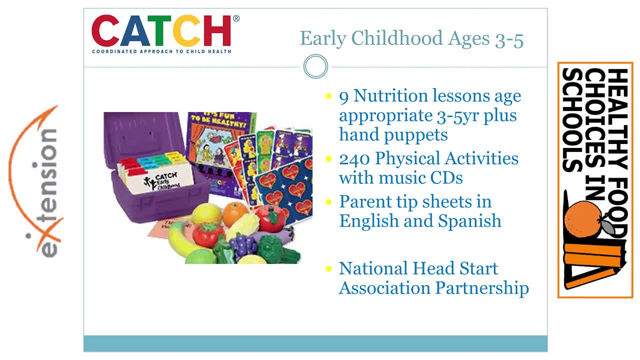 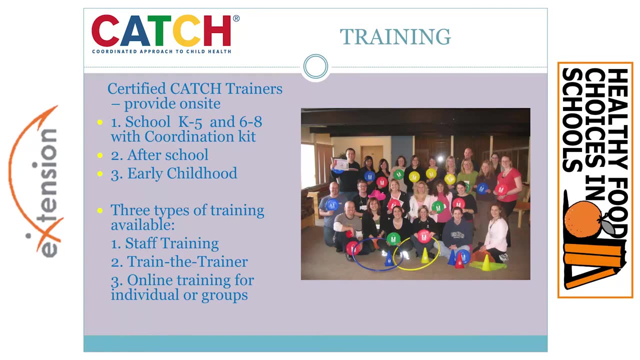 It includes age-appropriate a variety of learning activities. It uses music, stories, songs, hands-on activities and it has hand puppets that go with the nutrition lessons. Training is crucial and very important when implementing Catch And we have training for each. 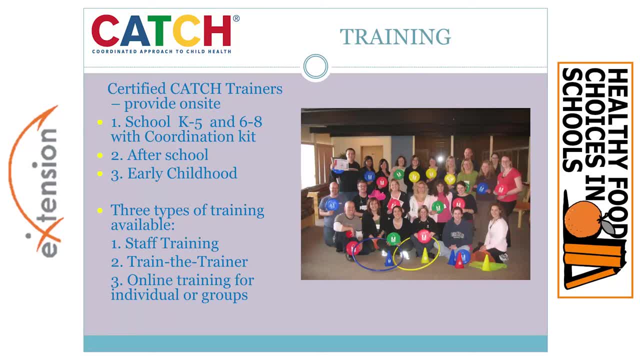 Of the Catch programs- the school-based, the after-school and the preschool- And there are three types of training per program. There's a staff training, where you can set up an employee staff trainer to come out and train a group of about 35 in one day. 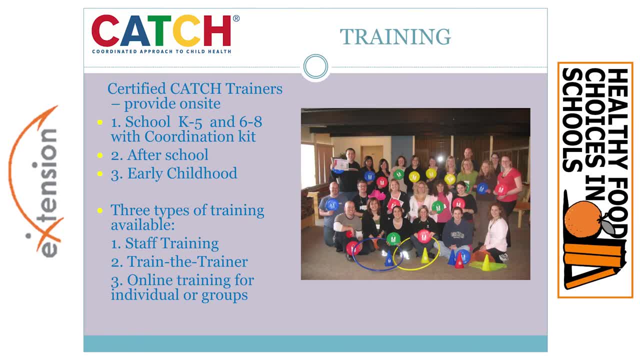 There is a three-day train-the-trainer where you can train a group of 35 in day one and then train about 15 over the day two, and three for your association to train others, And there is an online version of training for each of the programs. 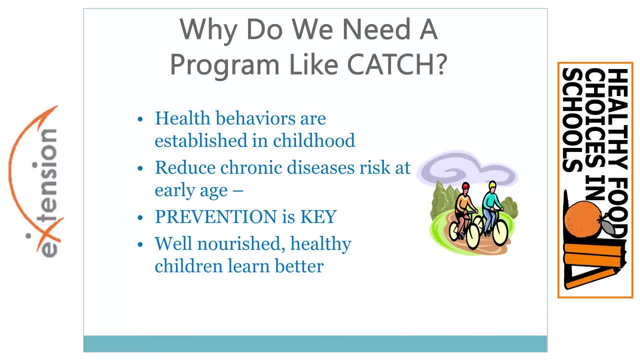 We do need a program like Catch because health behaviors are established in childhood. It's important to reduce chronic disease risk at a very early age. Prevention is key And we know well-nourished children learn better and it's crucial to impact their health behavior early. 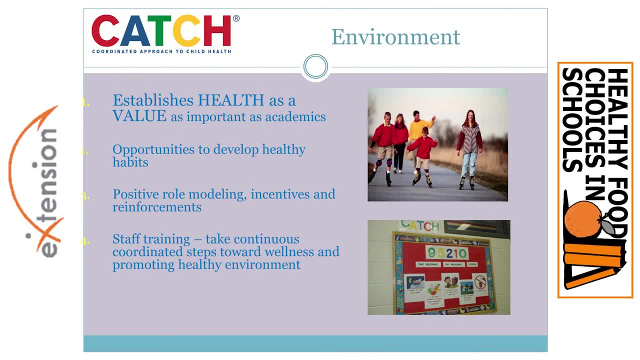 So, as far as the environment of Catch, it does establish health as a value, as equal to academics. It provides a curriculum base and plenty of opportunity to practice- Thank you- Participate and develop healthy habits. It gives you a format and reminds you of positive role modeling, incentives and reinforcements and lots of staff training opportunity. 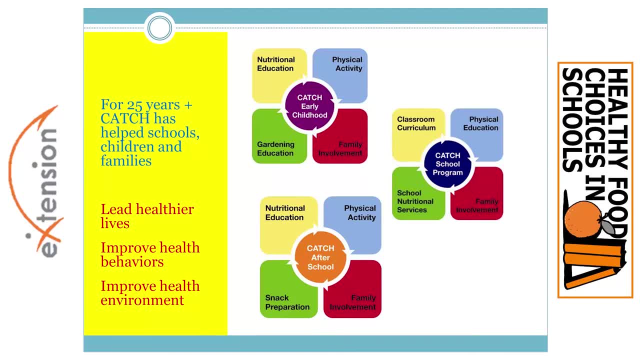 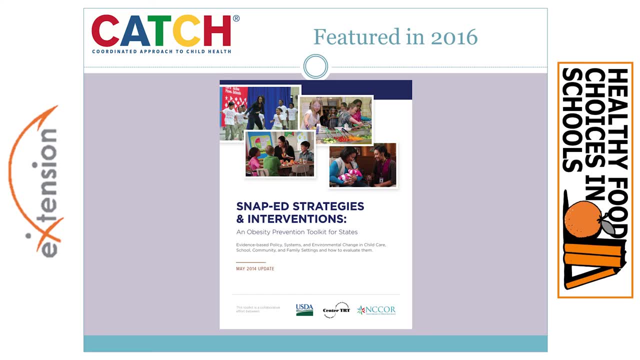 Catch has been at it about 25 years. There you see the different model parts: the early childhood, the school-based and the after-school program. The USDA reviewed Catch and Catch is now listed in the USDA SNAP-Ed Interventions Toolkit for States. 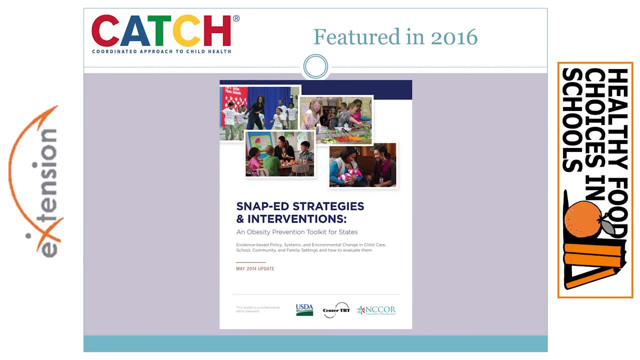 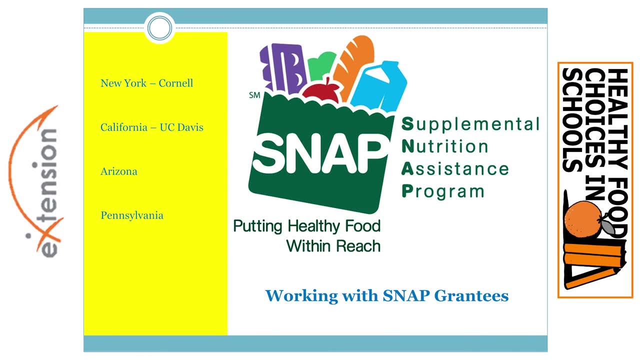 I have worked with several states Looking to adopt and several have adopted Catch when crafting their nutrition and physical activity plans. There is a few I know. New York State Cornell has been active now about two years or so. California, UC Davis is utilizing Catch.